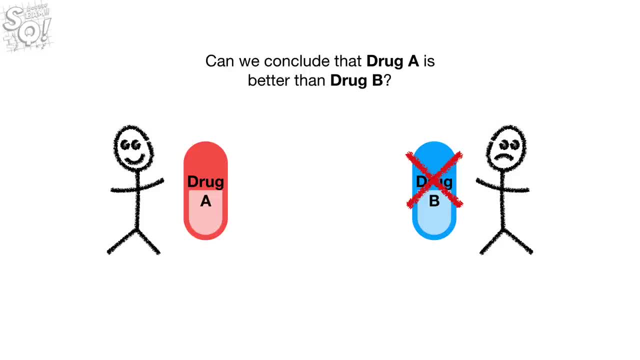 Bummer, Can we conclude that drug A is better than drug B? Nope, Drug B may have failed for a lot of people For a lot of different reasons. Maybe this guy is taking a medication that has a bad interaction with drug B. Or maybe this guy has a rare allergy to drug B. Or maybe this guy didn't take drug B properly and missed a dose. Or maybe drug A doesn't actually work and the placebo effect deserves all of the credit. There are a lot of weird, random things that can happen when doing a test. 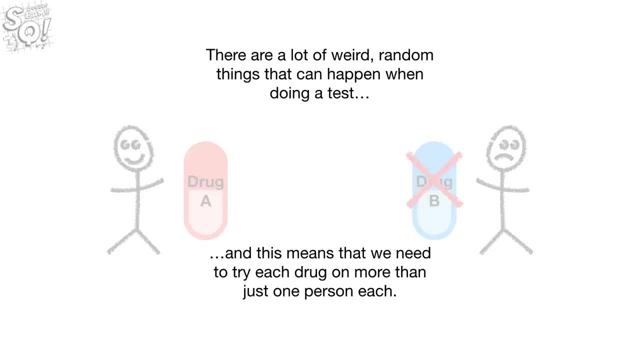 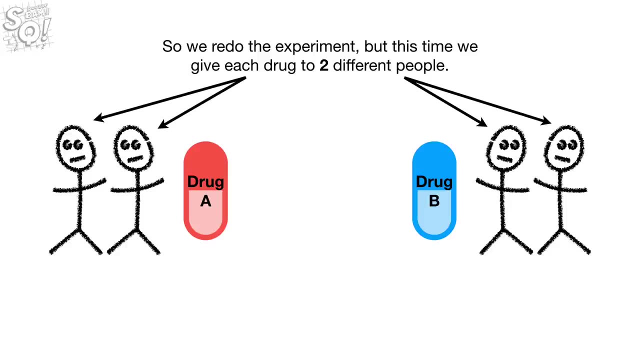 And this means that we need to try each drug on more than just one person each. So we redo the experiment, But this time we give each drug to two different people. This time, both people taking drug A are cured- Hooray. 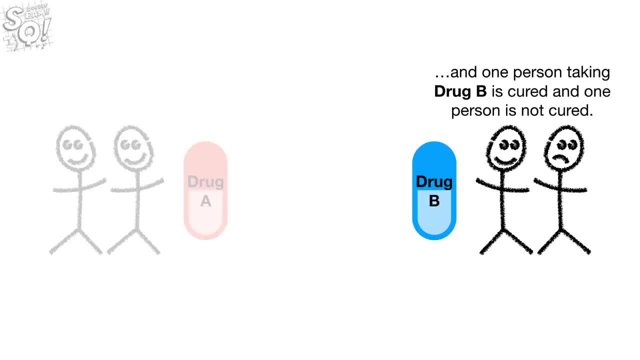 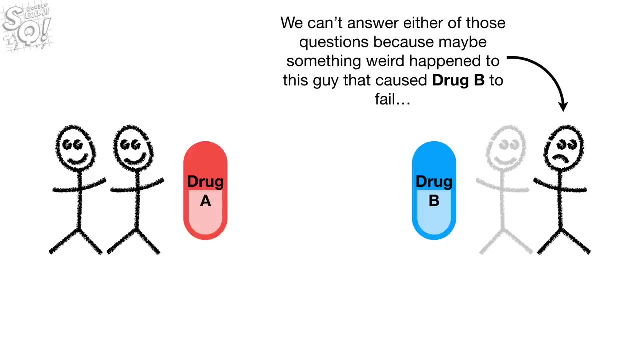 And one person taking drug B is cured and one person is not cured? Hooray And bummer, Is drug A better? Are both drugs the same? We can't answer either of those questions, because maybe something weird happened to this guy that caused drug B to fail. 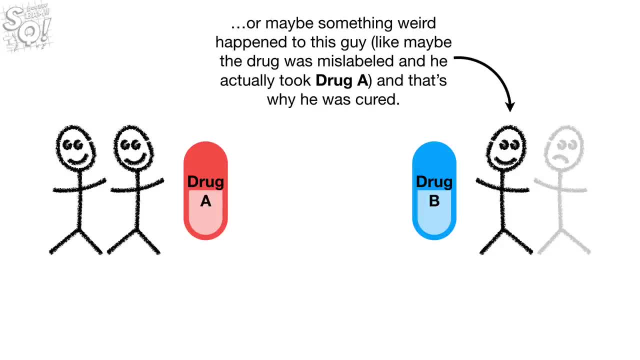 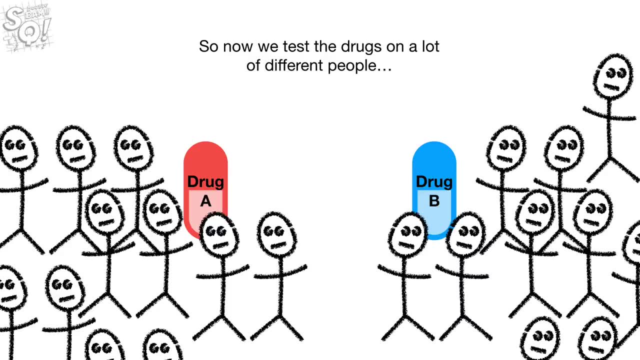 Or maybe something weird happened to this guy, Like maybe the drug was mislabeled and he actually took drug A And that's why he was cured. So now we test the drugs on a lot of different people And these are the results. 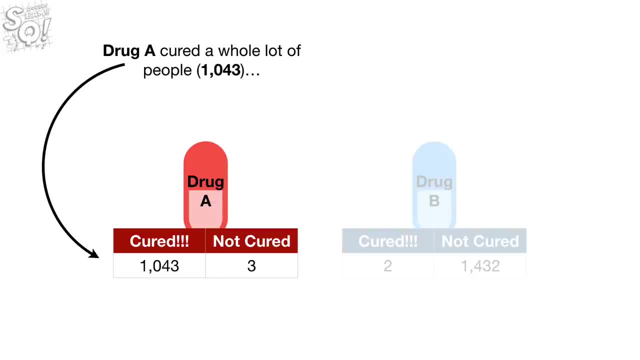 Drug A cured a whole lot of people: 1,043.. Compared to the number of people it didn't cure: 3.. In other words, 99.7% of the 1,046 people using drug A were cured. In contrast, drug B only cured a few people. 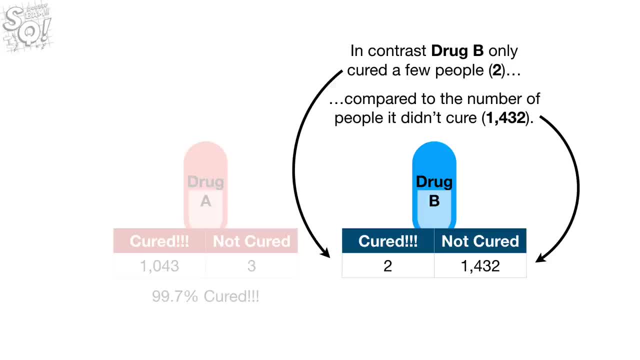 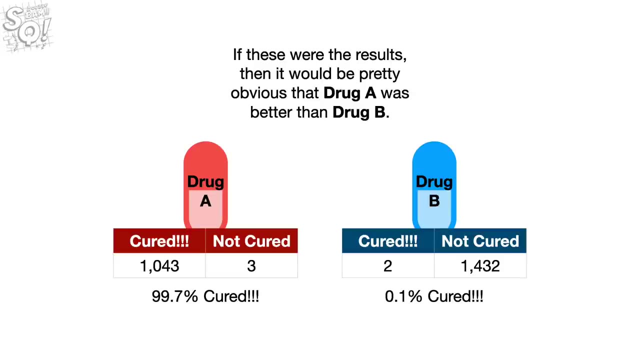 2., 3. In other words, only 0.1% of the 1,434 people using drug B were cured. If these were the results, then it would be pretty obvious that drug A was better than drug B. In other words, it would seem unrealistic to suppose that these results were cured. 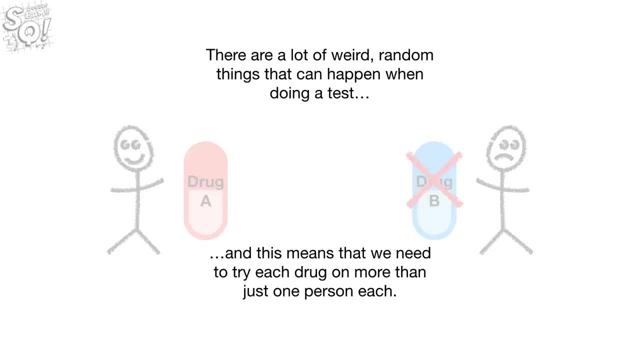 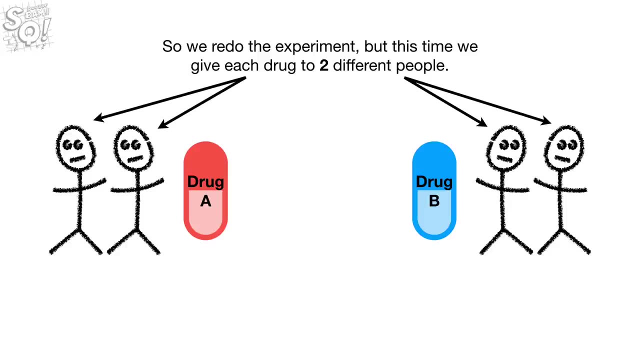 And this means that we need to try each drug on more than just one person each. So we redo the experiment, But this time we give each drug to two different people. This time, both people taking drug A are cured- Hooray. 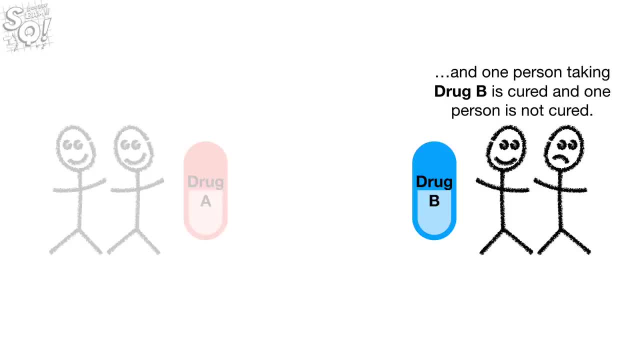 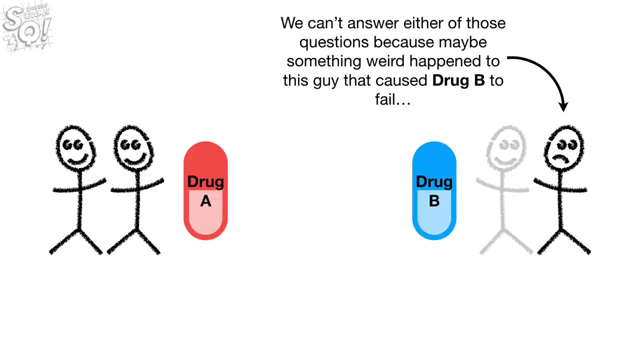 And one person taking drug B is cured and one person is not cured? Hooray And bummer, Is drug A better? Are both drugs the same? We can't answer either of those questions, because maybe something weird happened to this guy that caused drug B to fail. 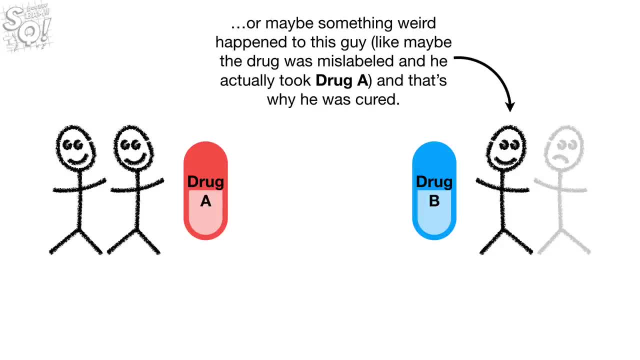 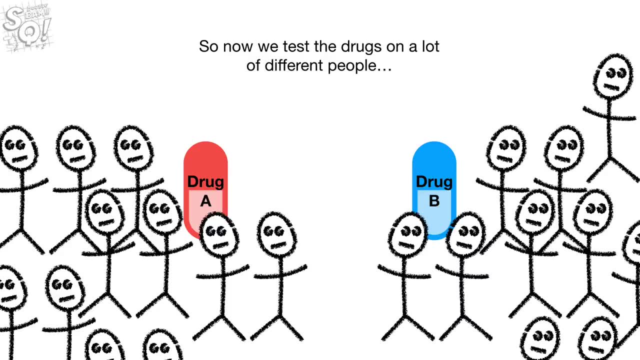 Or maybe something weird happened to this guy, Like maybe the drug was mislabeled and he actually took drug A And that's why he was cured. So now we test the drugs on a lot of different people And these are the results. 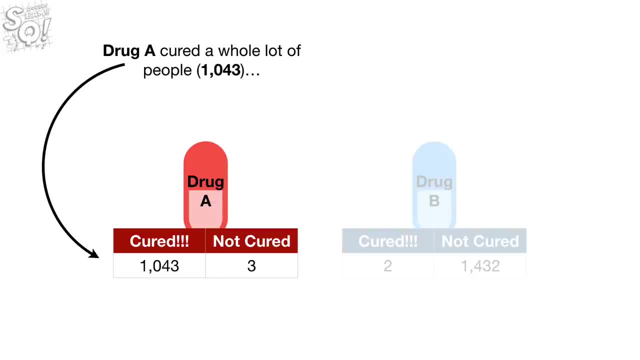 Drug A cured a whole lot of people: 1,043.. Compared to the number of people it didn't cure: 3.. In other words, 99.7% of the 1,046 people using drug A were cured. In contrast, drug B only cured a few people. 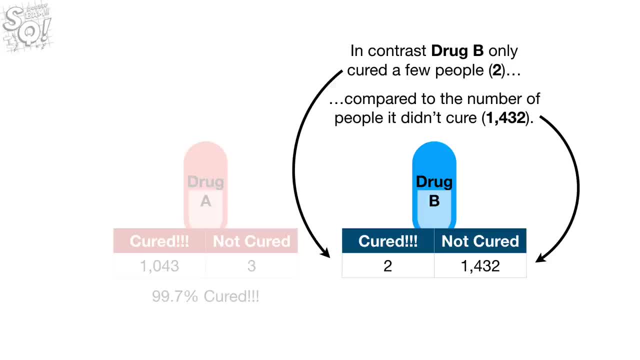 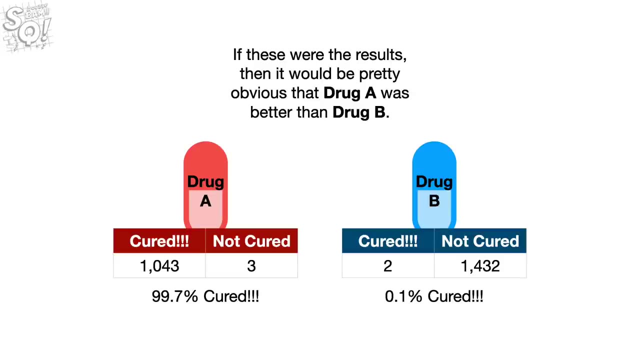 2., 3. In other words, only 0.1% of the 1,434 people using drug B were cured. If these were the results, then it would be pretty obvious that drug A was better than drug B. In other words, it would seem unrealistic to suppose that these results were cured. 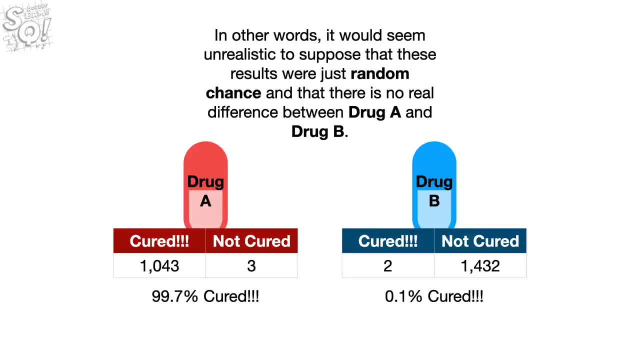 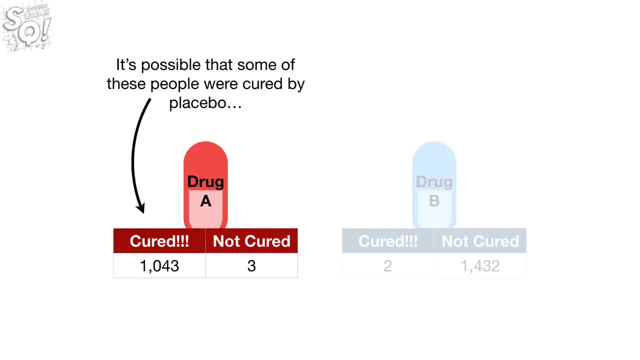 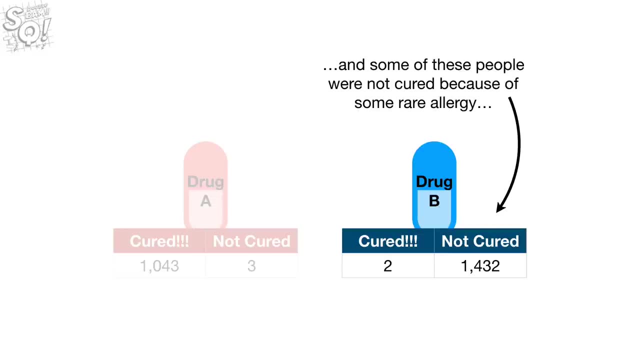 They are just random chance and that there is no real difference between drug A and drug B. It's possible that some of these people were cured by placebo And some of these people were not cured because of some rare allergy, But there are just too many people cured by drug A and too few cured by drug B. 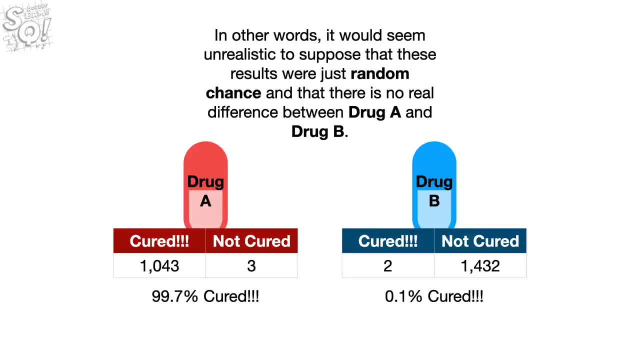 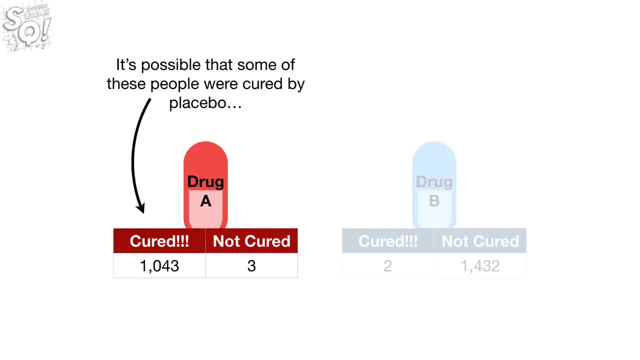 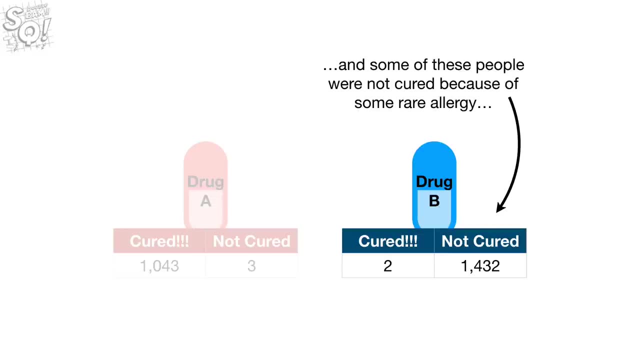 They are just random chance and that there is no real difference between drug A and drug B. It's possible that some of these people were cured by placebo And some of these people were not cured because of some rare allergy, But there are just too many people cured by drug A and too few cured by drug B. 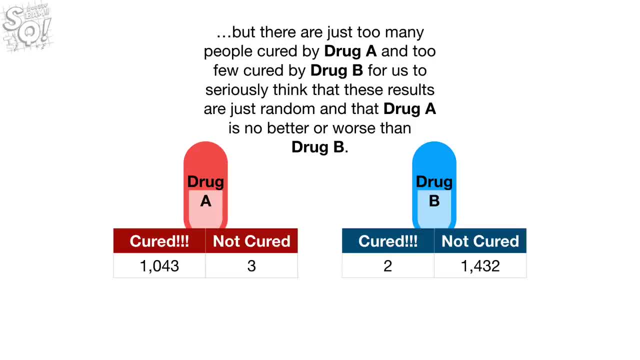 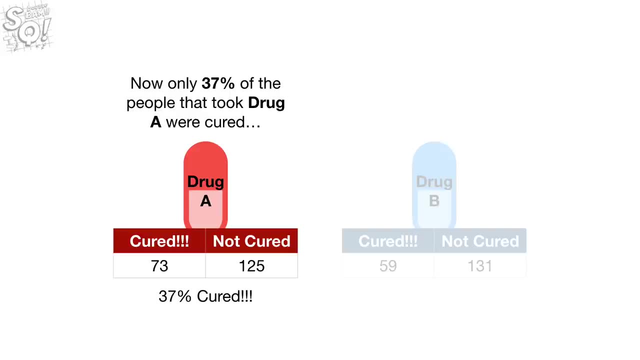 for us to seriously think that these results are just random and that drug A is no better Or worse than drug B. In contrast, what if these were the results Now? only 37% of the people that took drug A were cured. 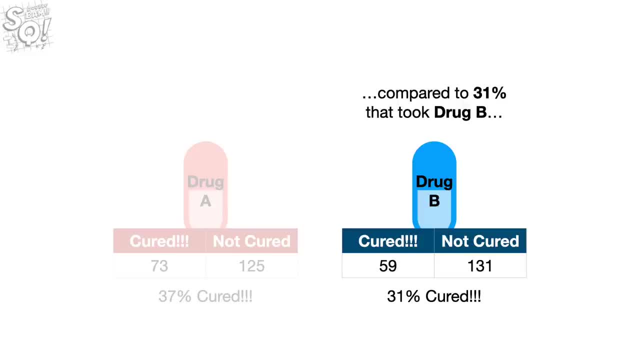 Compared to 31% that took drug B. So drug A cured a larger percentage of people. But, given that no study is perfect and there are always a few random things that happen, and there are always a few random things that happen, and there are always a few random things that happen- 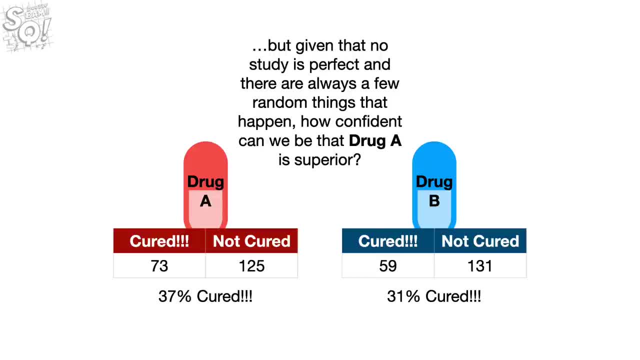 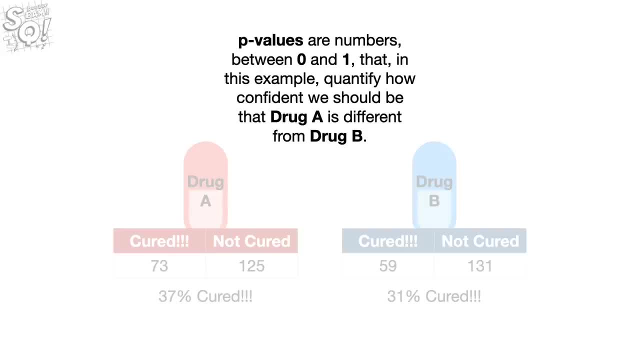 confident can we be that drug A is superior? That's where the p-value comes in. P-values are numbers between 0 and 1 that, in this example, quantify how confident we should be that drug A is different from drug B. The closer a p-value is to 0, the more confidence we have. 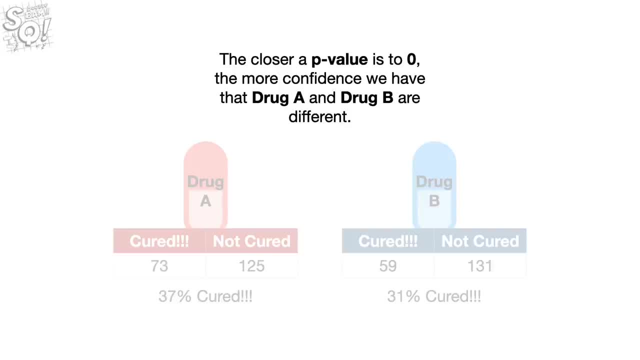 that drug A and drug B are different. So the question is: how small does a p-value have to be before we are sufficiently confident that drug A is different from drug B? In other words, what threshold can we use to make a good decision? 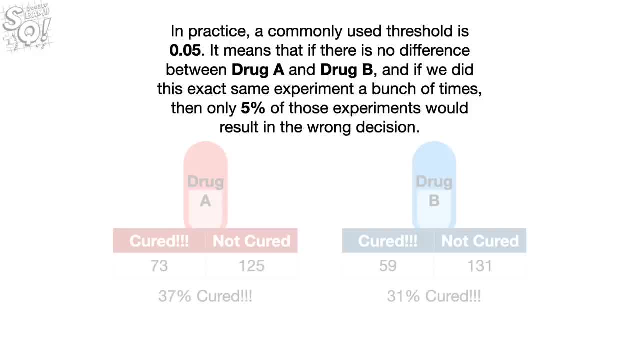 In practice. a commonly used threshold is 0.05.. It means that if there is no difference between drug A and drug B, there is no difference between drug A and drug B In practice. a commonly used threshold is 0.05.. It means that if there is no difference between drug A and drug B, 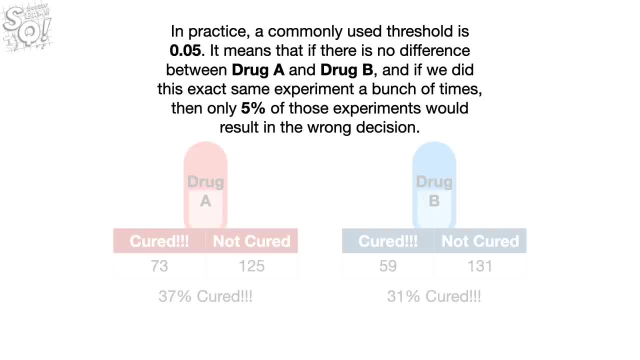 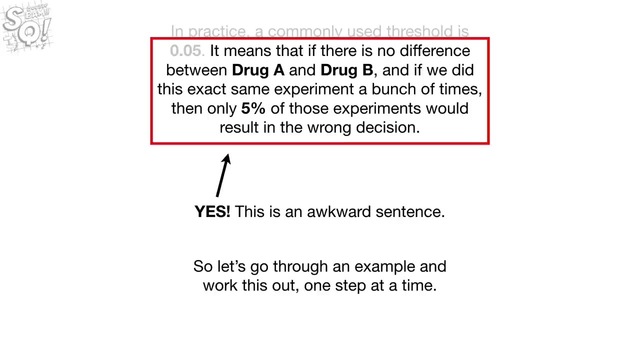 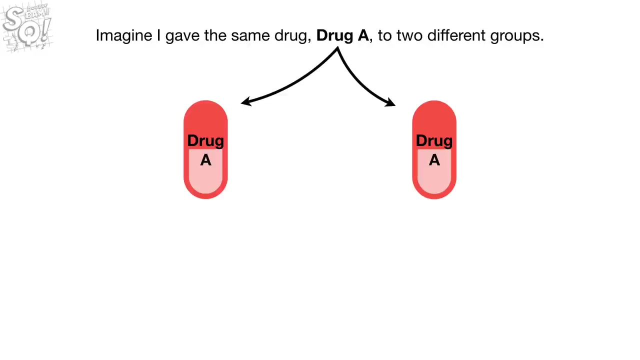 and if we did this exact same experiment a bunch of times, then only 5% of those experiments would result in the wrong decision. Yes, this is an awkward sentence, So let's go through an example and work this out one step at a time. Imagine I gave the same drug, drug A, to two different groups. Now any difference. 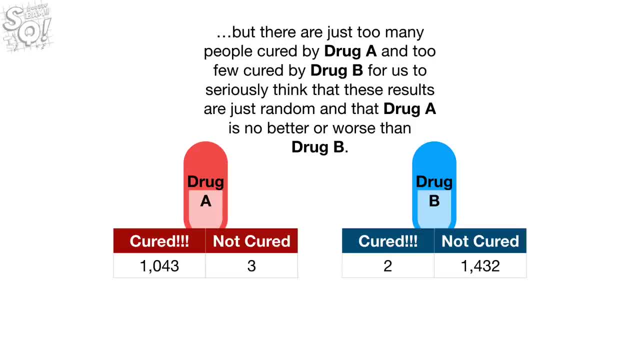 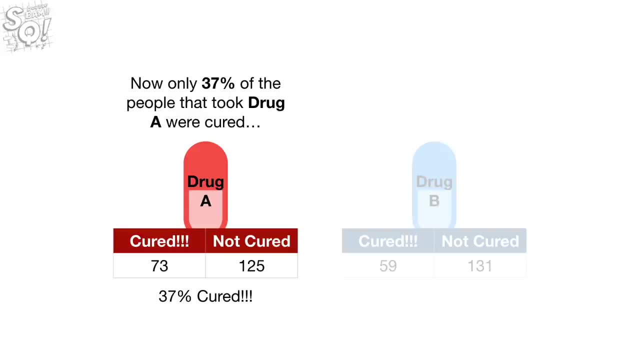 for us to seriously think that these results are just random and that drug A is no better. In contrast. what if these were the results Now? only 37% of the people that took drug A were cured, Compared to 31% that took drug B. 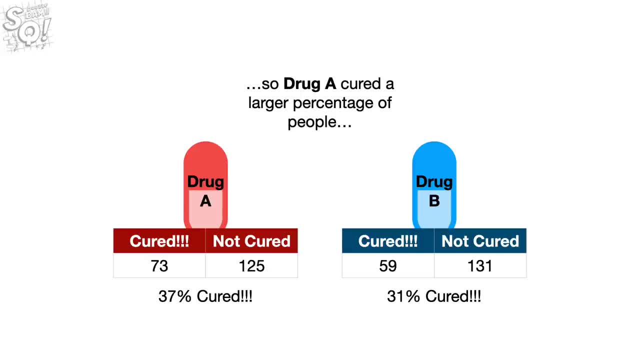 So drug A cured a larger percentage of people. But given that no study is perfect and there are always a few random things that happen, how confident can you be that drug A is cured? How confident can you be that drug A is cured? How confident can you be that drug A is cured? 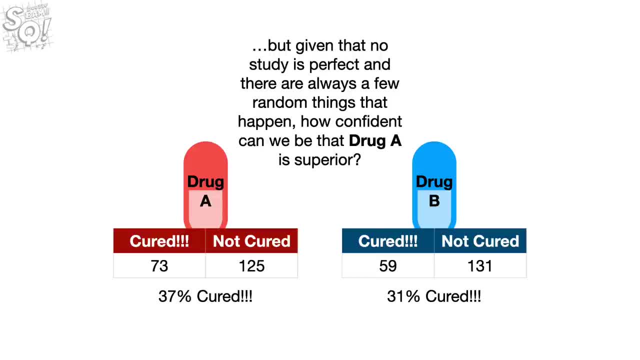 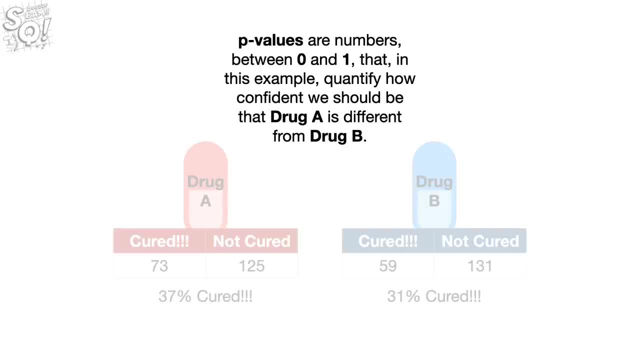 How confident can we be that drug A is superior? That's where the p-value comes in. P-values are numbers between 0 and 1 that, in this example, quantify how confident we should be that drug A is different from drug B. 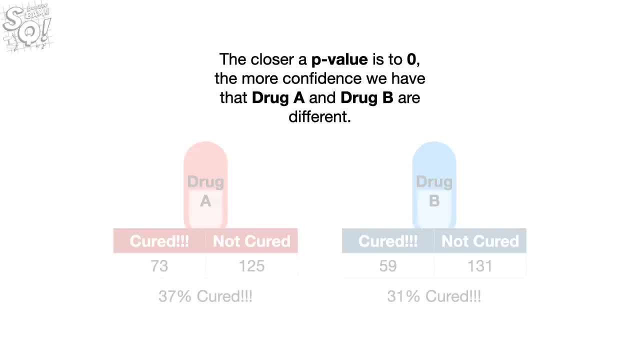 The closer a p-value is to 0,, the more confidence we have that drug A and drug B are different. So the question is: how small does a p-value have to be before we are sufficiently confident that drug A is different from drug B? 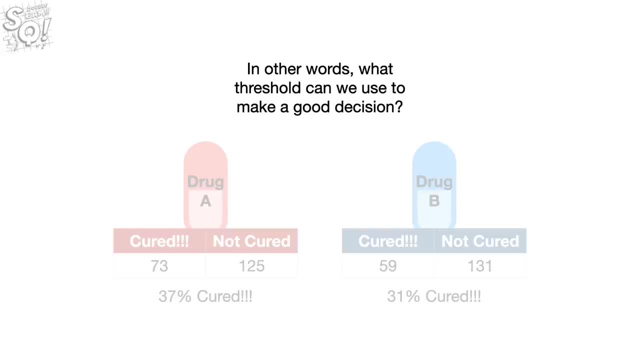 In other words, what threshold can we use to make a good decision In practice? a commonly used threshold is 0.05.. It means that if there is no difference between drug A and drug B and if we did this exact same experiment a bunch of times, 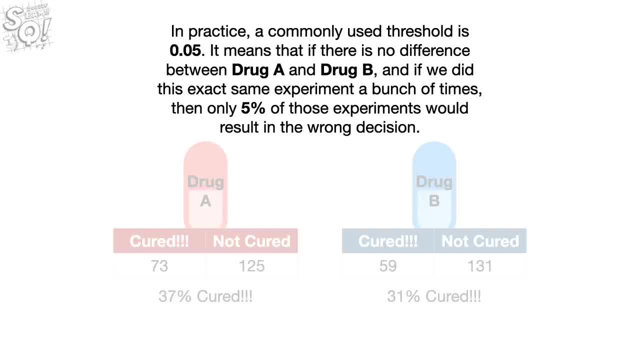 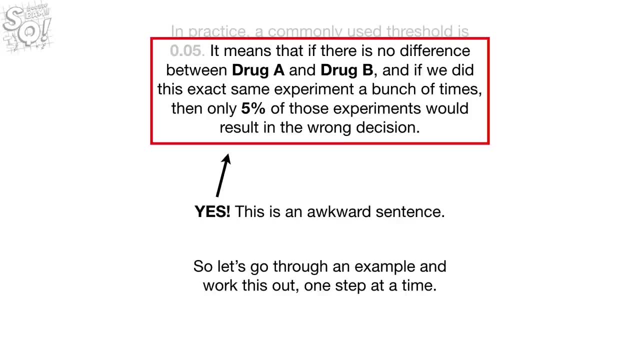 then only 4% of the people that took drug A are cured, And only 5% of those experiments would result in the wrong decision. Yes, this is an awkward sentence, So let's go through an example and work this out one step at a time. 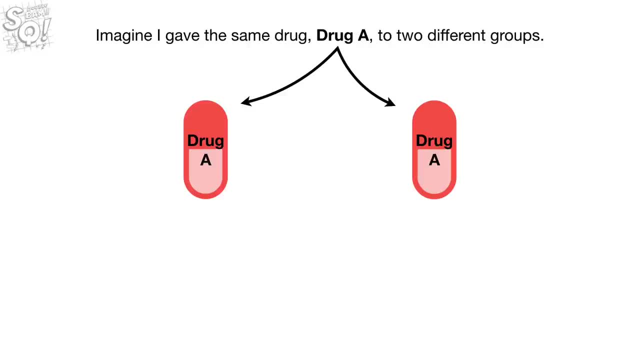 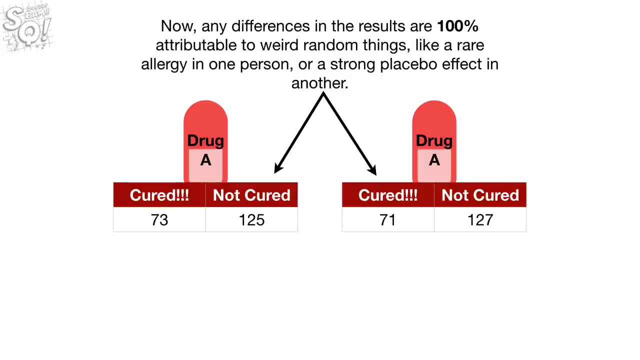 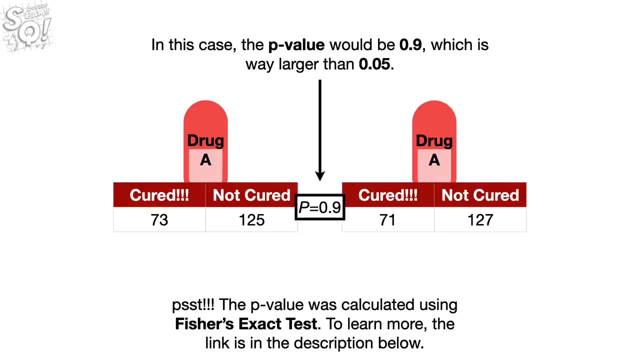 Imagine I gave the same drug- drug A- to two different groups. Now any differences in the results are 100% attributable to weird random things Like a rare allergy in one person or a strong placebo effect in another. In this case, the p-value would be 0.9,, which is way larger than 0.05.. 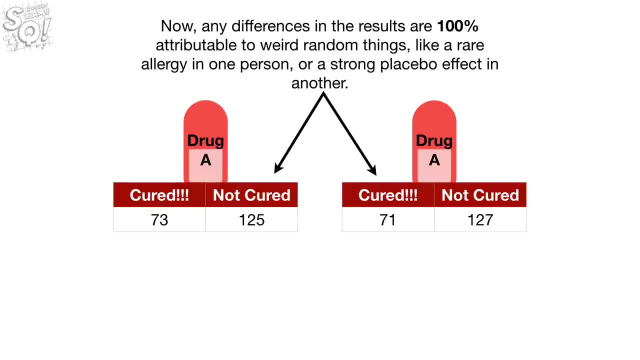 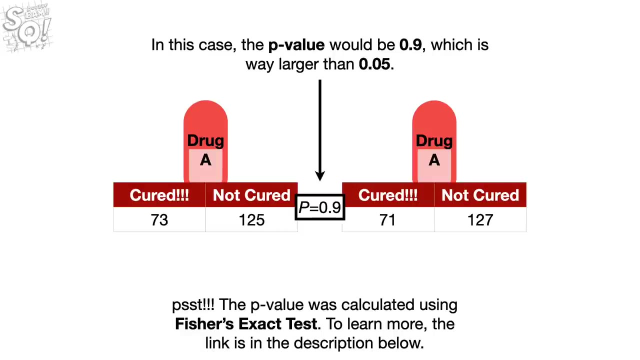 in the results are 100% attributable to weird random things like a rare allergy in one person or a strong placebo effect in another. In this case, the p-value would be 0.9,, which is way larger than 0.05.. Thus, we would say that we fail to see a difference. 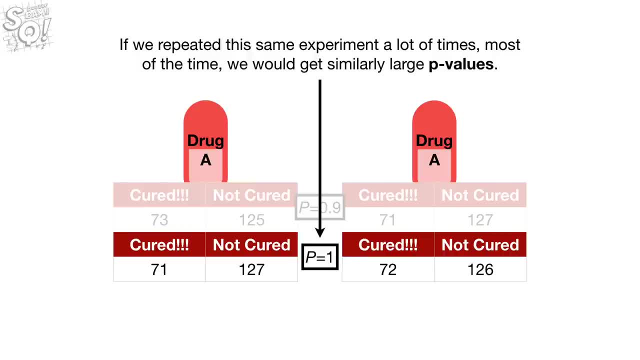 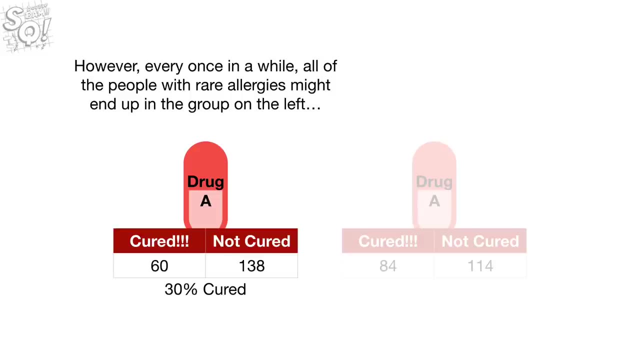 between the two groups. If we repeated this same experiment a lot of times, most of the time we would get similarly large p-values. However, every once in a while, all of the people with rare allergies might end up in the group on the left. 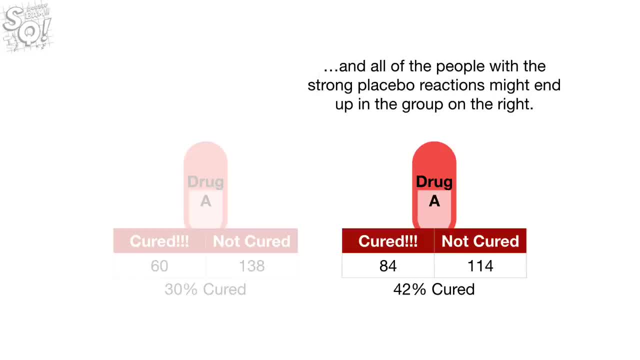 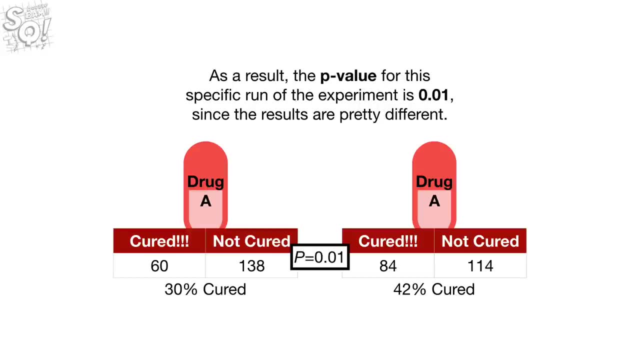 and all of the people with the strong placebo reactions might end up in the group on the right. As a result, the p-value for this specific run of the experiment is 0.01, since the results are pretty different. Thus, in this case, we would say that the two groups are different, even though they 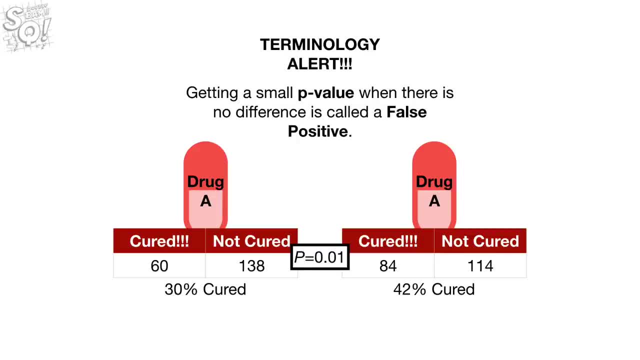 both took the same drug. Oh no, it's the dreaded terminology alert. Getting a small p-value when there is no difference is called a false positive. A 0.05 threshold for p-values means that 5% of the experiments where the only differences 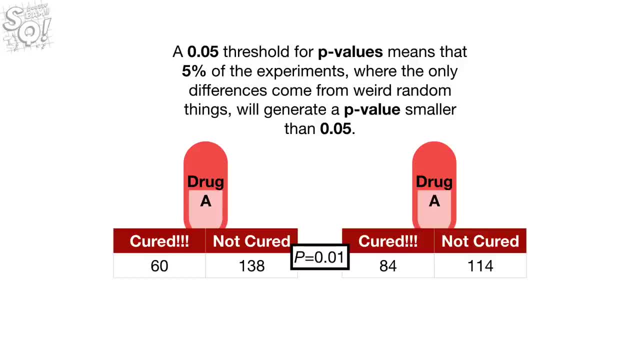 come from weird random things will generate a p-value smaller than 0.05.. In other words, if there is no difference between drug A and drug B, 5% of the time we do the experiment, we will get a p-value less than 0.05, aka a false positive. 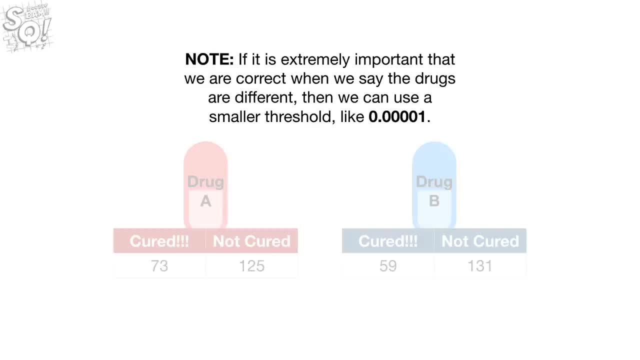 If it is extremely important that we are correct when we say the drugs are different, then we can use a p-value. We can use a smaller threshold, like 0.00001.. Using a threshold of 0.00001 means we would only get a false positive once every 100,000. 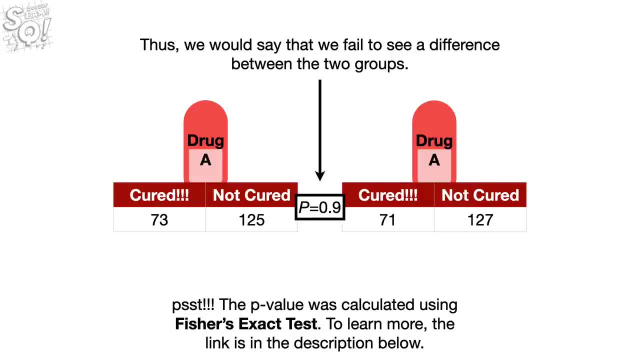 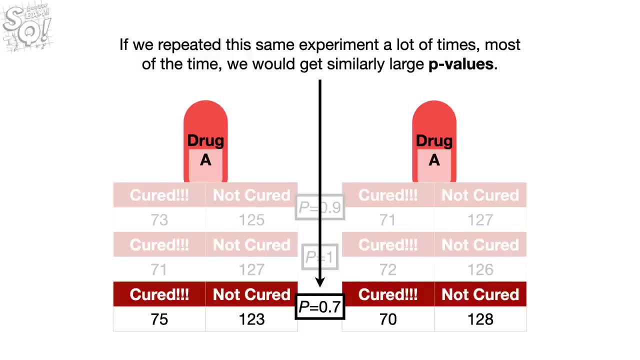 Thus, we would say that we fail to see a difference between the two groups. If we repeated this same experiment a lot of times, most of the time we would get similarly large p-values. However, if we repeated this experiment a lot of times, 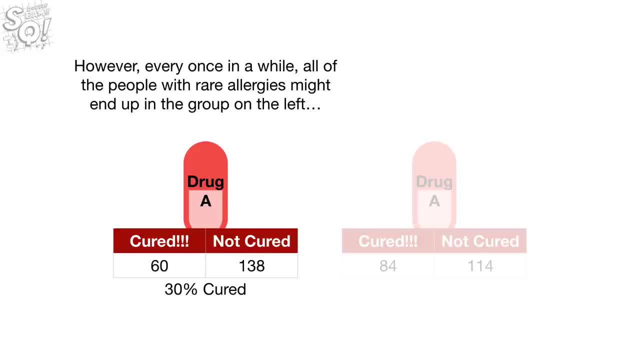 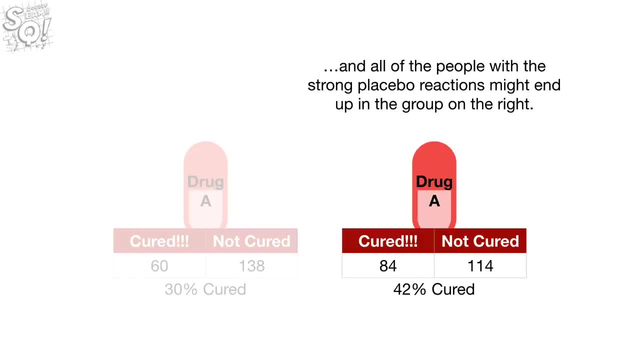 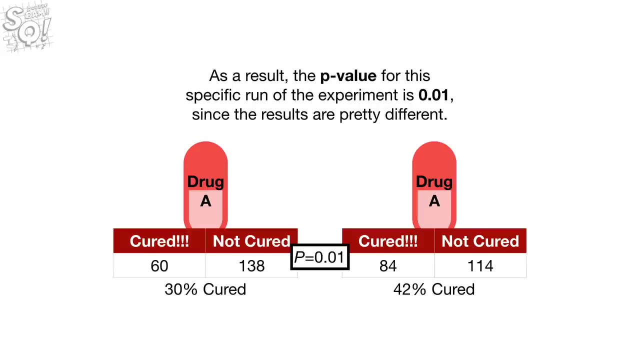 every once in a while, all of the people with rare allergies might end up in the group on the left And all of the people with the strong placebo reactions might end up in the group on the right. As a result, the p-value for this specific run of the experiment is 0.01,. 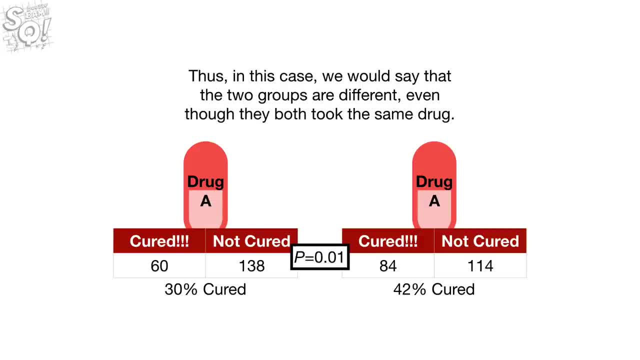 since the results are pretty different. Thus, in this case, we would say that the two groups are different, even though they both are different, Even though they both took the same drug. Oh no, It's the dreaded terminology alert. Getting a small p-value when there is no difference is called a false positive. 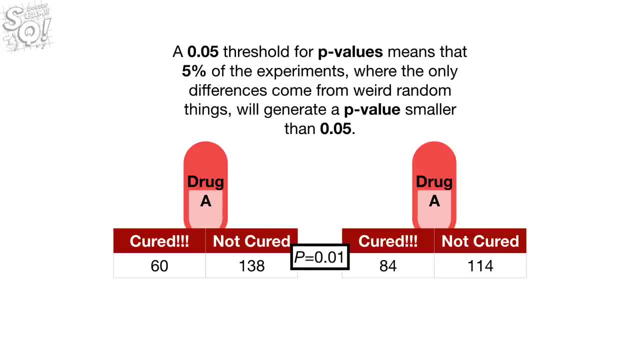 A 0.05 threshold for p-values means that 5% of the experiments where the only differences come from weird, random things will generate a p-value smaller than 0.05.. In other words, if there is no difference between drug A and drug B, 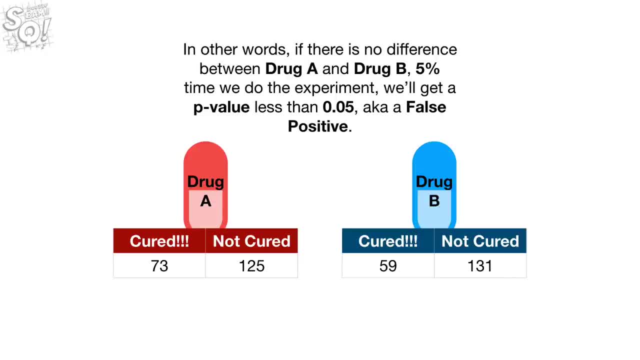 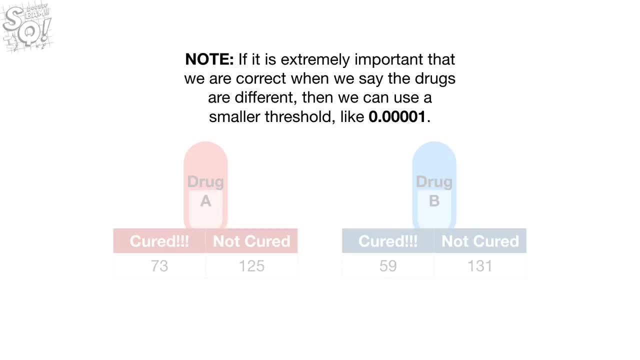 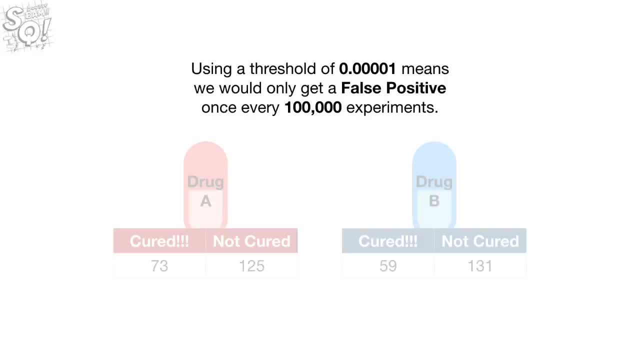 Using a threshold like 0.000001, we can get a p-value of 0.000001.. Using a threshold like 0.000001,, we can get a p-value of 0.000001.. means we would only get a false positive once every 100,000 experiments. 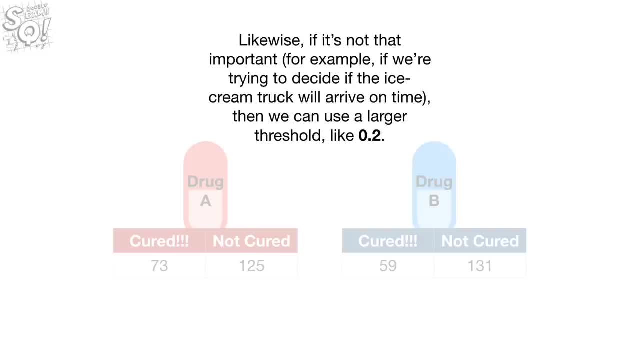 experiments. Likewise, if it's not that important- for example, if we're trying to decide if the ice cream truck will arrive on time- then we can use a larger threshold like 0.0001.. Using a threshold of 0.00002 means we are willing to get a false positive 2 times out. 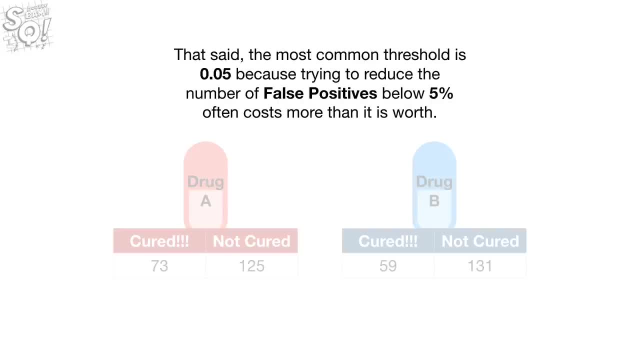 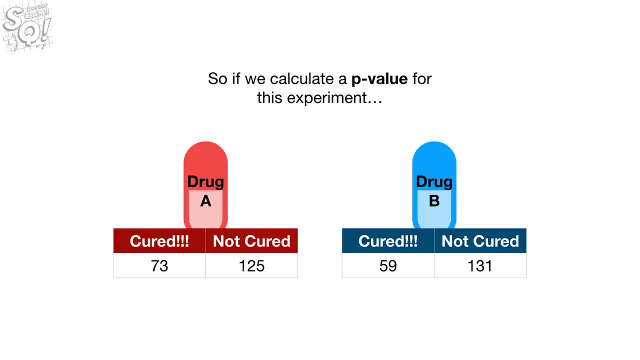 of 10.. That said, the most common threshold is 0.005, because trying to reduce the number of false positives below 5% often costs more than it's worth. So if we calculate a p-value for this experiment…. …and the p-value is less than 0.001…. 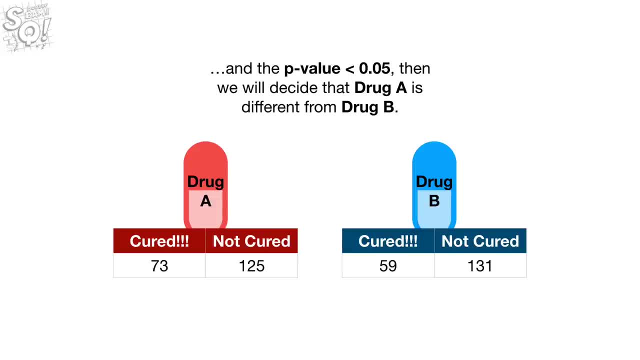 …then we can calculate a p-value for this experiment…. …and if the p-value is less than 0.005, then we will decide that drug A is different from drug B. That said, the p-value is actually 0.24, so we are not confident that drug A is different. 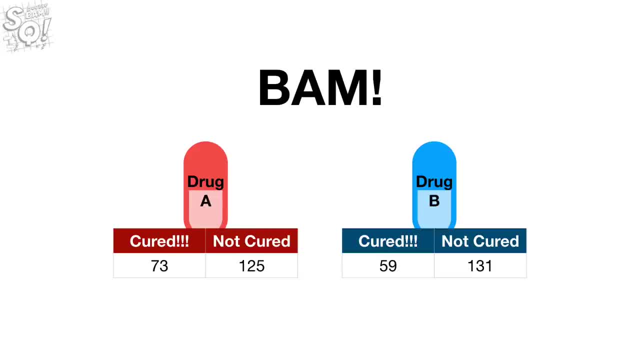 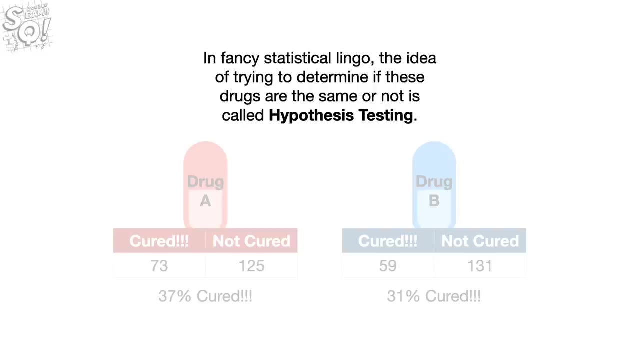 from drug B Bam. Okay, before we're done, let me say two more things about p-values. Unfortunately, the first thing I want to say is just more terminology In fancy statistical lingo, the idea of trying to determine if these drugs are the same. 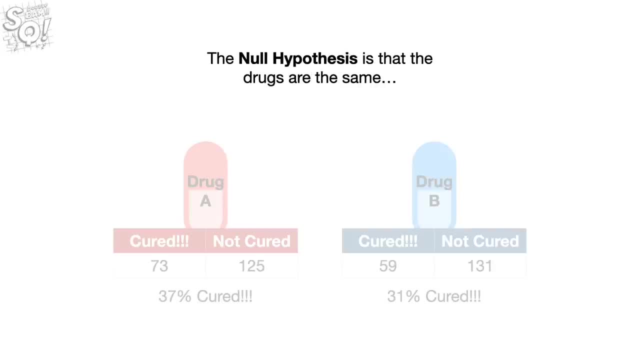 or not is called hypothesis testing. The null hypothesis is that the drugs are the same And the p-value helps us decide if we should reject the null hypothesis or not. Small bam, Okay. Now that we have that fancy terminology out of the way…. 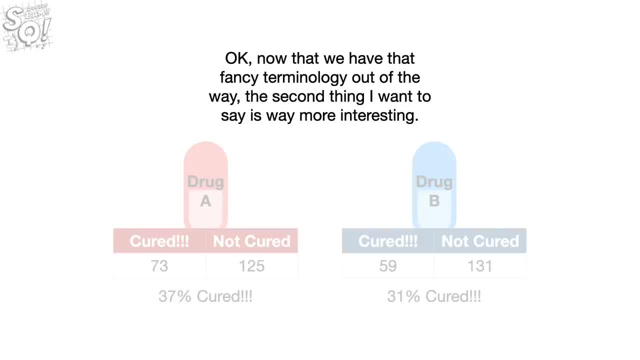 …the second thing I want to say is way more interesting. While a small p-value helps us decide if drug A is different from drug B, it does not tell us how different they are. In other words, you can have a small p-value regardless of the size of difference between. 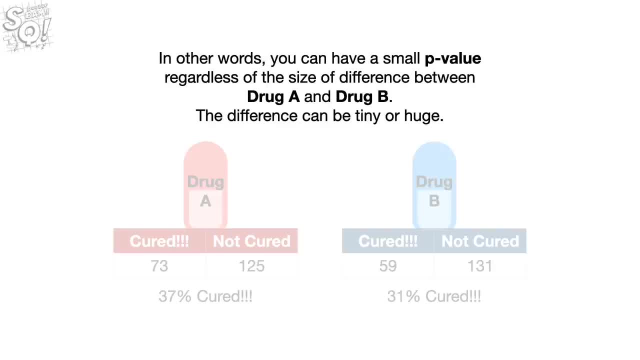 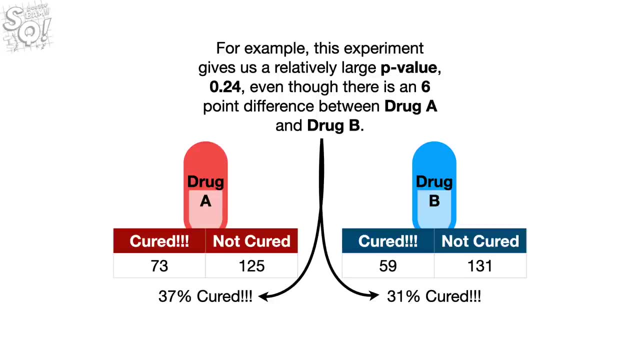 drug A and drug B. The difference can be tiny or huge. For example… …this experiment… …gives us a relatively large p-value… …0.24… …even though there is a 6-point difference between drug A and drug B. 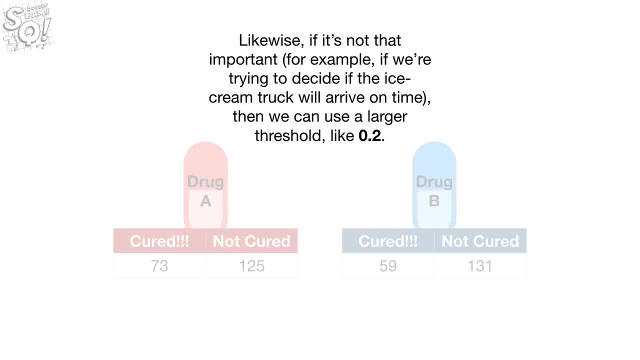 Likewise, if it's not that important- for example, if we're trying to decide if the ice cream truck will arrive on time- then we can use a larger threshold like 0.2.. Using a threshold of 0.2 means we are willing to get a false positive two times out of 10.. 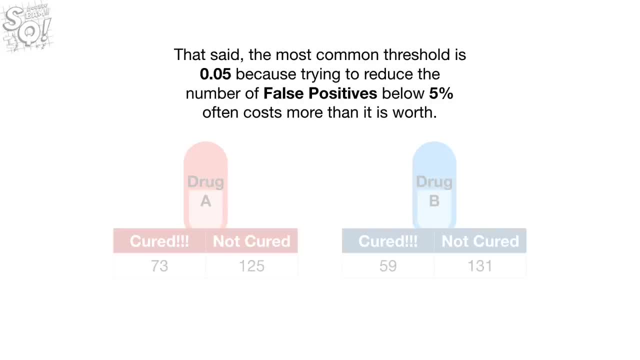 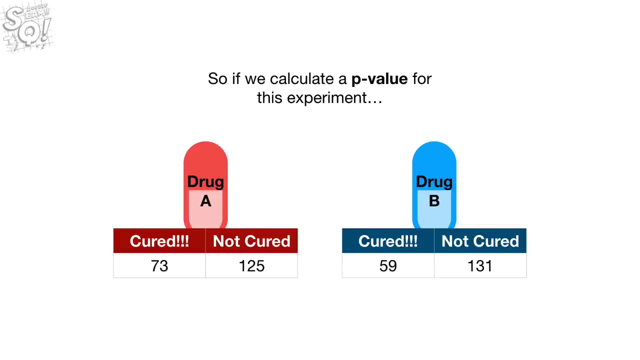 That said, the most common threshold is 0.05, because trying to reduce the number of false positives below 5% often costs more than it's worth. So if we calculate a p-value for this experiment and the p-value is less than 0.05,, 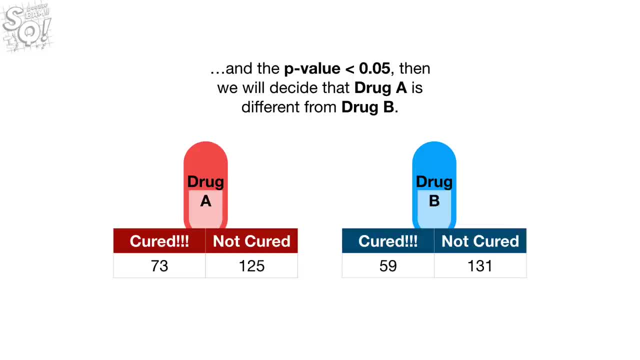 then we will decide that drug A is different from drug B. That said, the p-value is 0.05, and the p-value is actually 0.24, so we are not confident that drug A is different from drug B Bam. 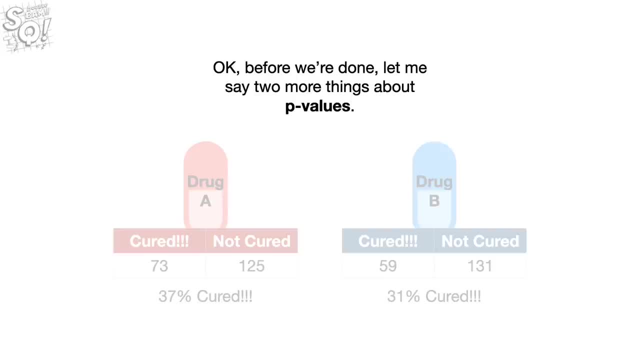 Okay, before we're done, let me say two more things about p-values. Unfortunately, the first thing I want to say is just more terminology. In fancy statistical lingo, the idea of trying to determine if these drugs are the same or not is called hypothesis testing. 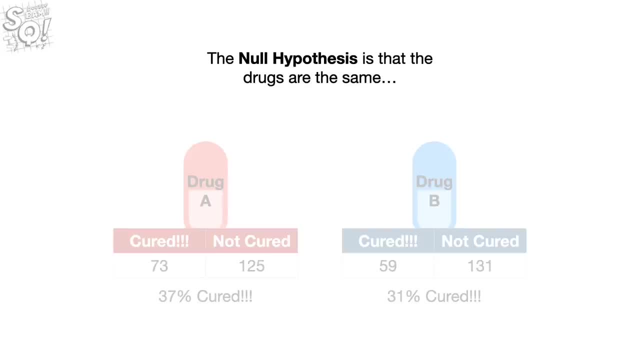 The null hypothesis is that the drugs are the same and the p-value helps us decide if we should reject the null hypothesis or not. Small bam, Okay, now that we have that fancy terminology out of the way, the second thing I want to say is way more interesting. 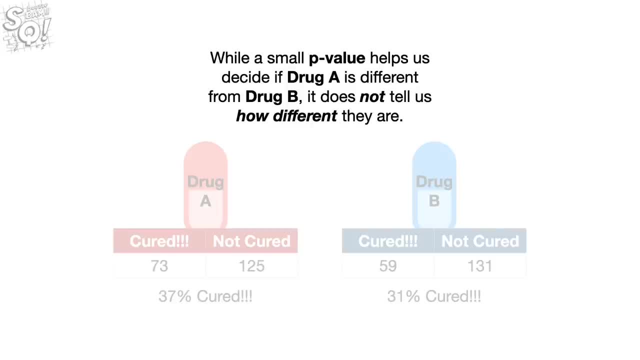 While a small p-value helps us decide if drug A is different from drug B, it does not depend on the p-value. It does not us how different they are. In other words, you can have a small p-value regardless of the size. 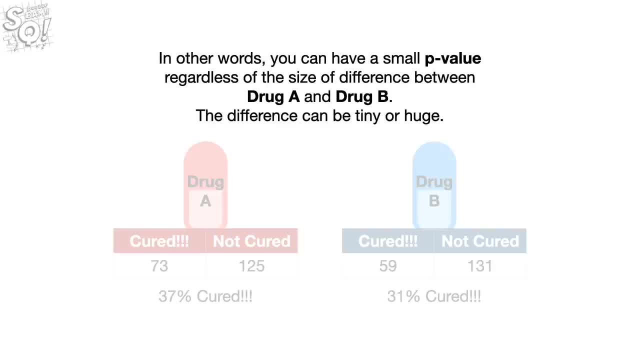 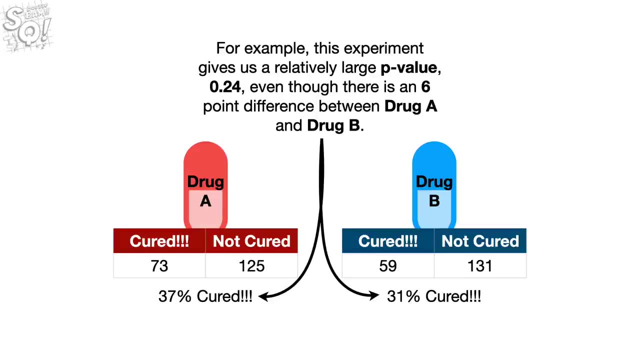 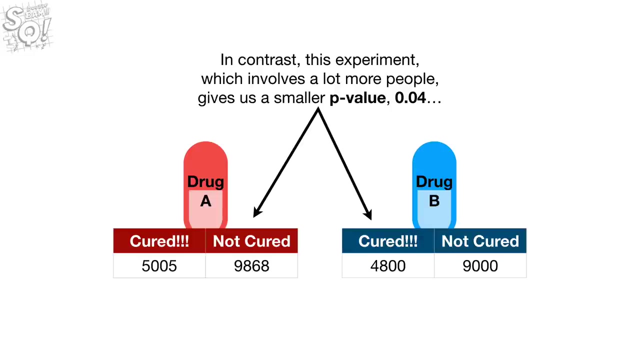 of difference between drug A and drug B. The difference can be tiny or huge. For example, this experiment gives us a relatively large p-value- 0.24, even though there is a six-point difference between drug A and drug B. In contrast, this experiment, which involves a lot more people,